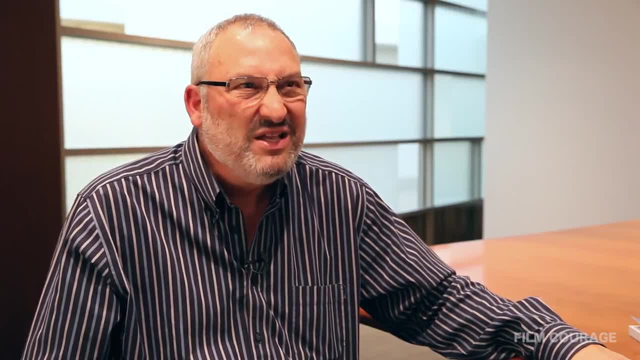 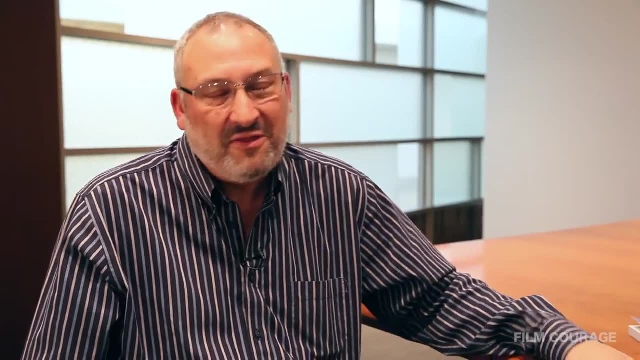 your characters, you're not growing your series And it's real easy for the audience to get tired of your show if it's sort of the same joke over and, over and over again, And I think this is why some characters are great series characters and others are standalone. I think the example I give in my book 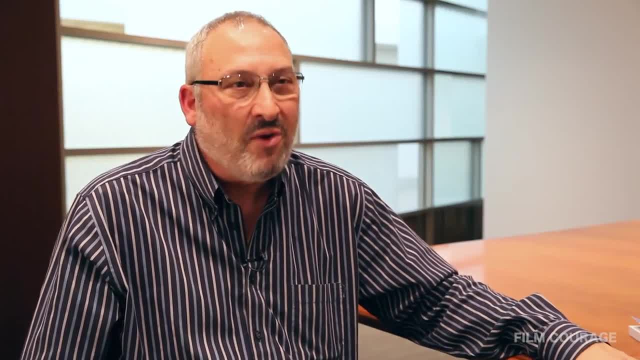 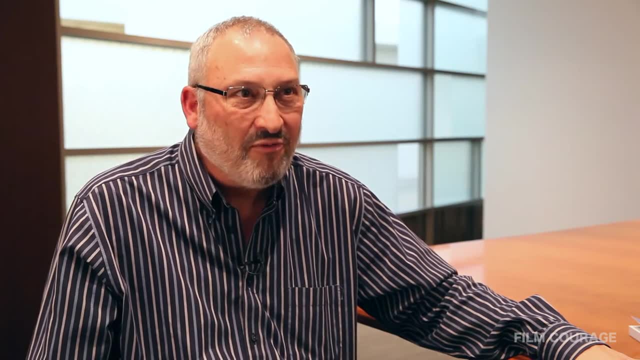 is that the soup Nazi on Seinfeld is a great character for a couple episodes, but you do not want to try and write the soup Nazi series because it's the same joke over and over again. You: no soup for two weeks. Or you say: well, what about on a date? It's going to be you. 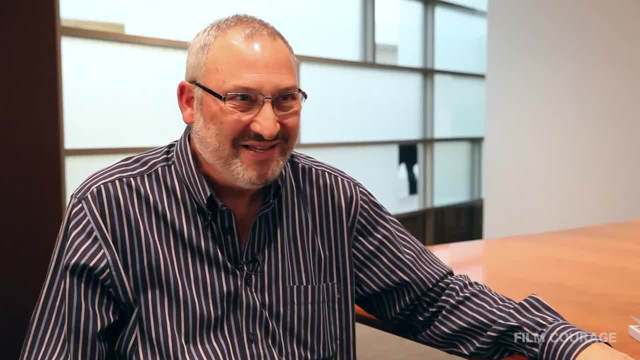 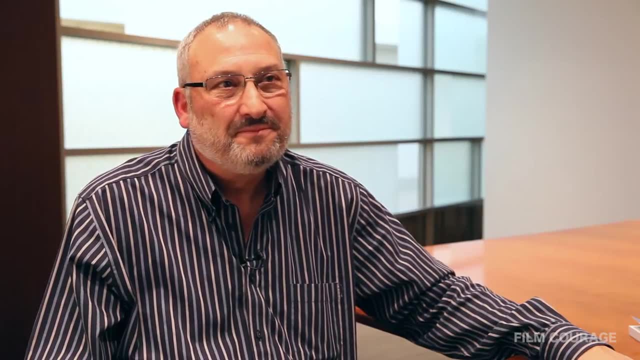 no date for two weeks. It's the same. I don't know where you go with the soup Nazi. He's not as developed a character as Seinfeld or Kramer or Elaine or George Film Courage. What can someone do to play around with this supposed main character? 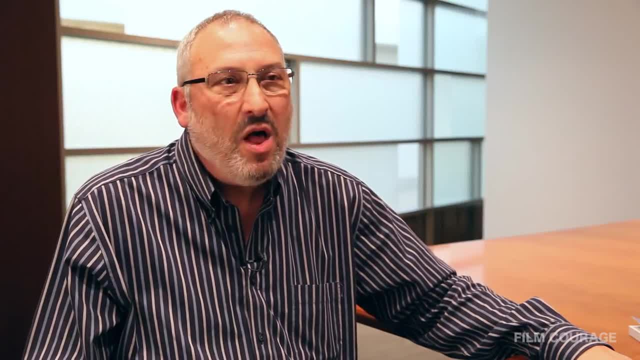 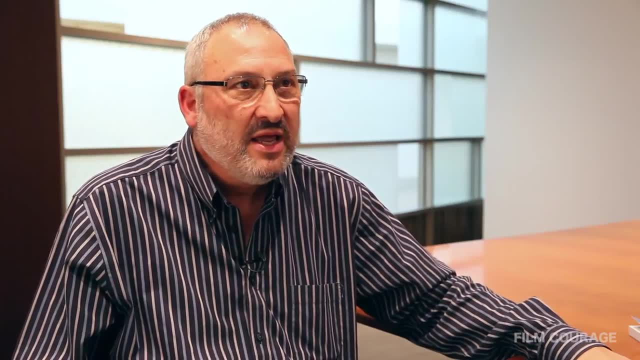 to see if they have legs, so to speak. Dr David Goldstein. Well, I think this is one of the things you should do while you're developing your series. and you're developing your pilot story is you should say: okay, what would future episodes be? You don't have to develop the whole story for it. 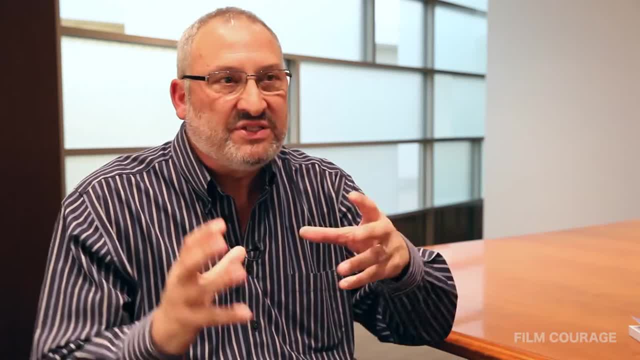 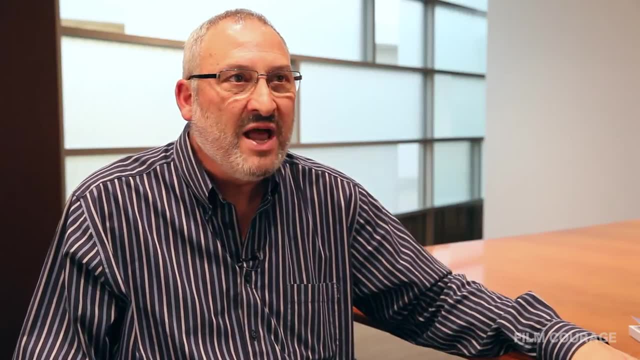 but what other situations can I put this character or this set of characters in? to get stories Again, just like in the traditional television world, you shoot a pilot for a network and they're going to evaluate it. You have to submit a half a dozen. 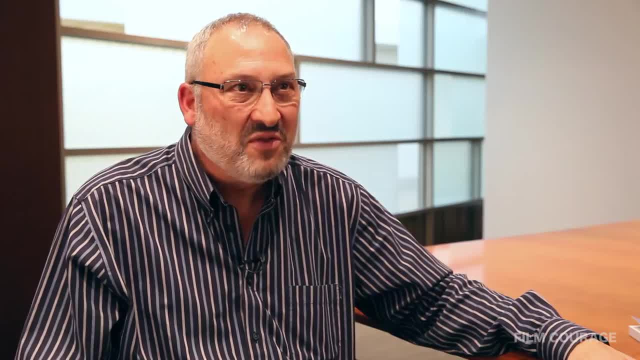 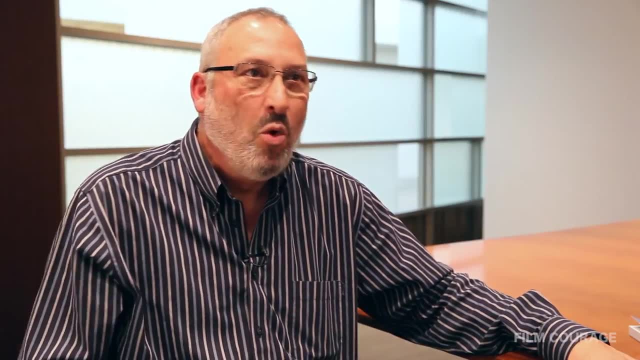 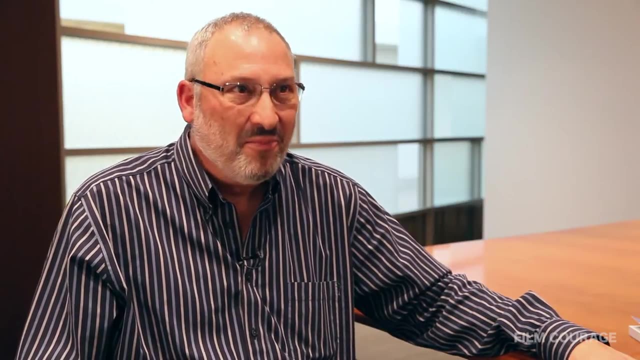 story ideas for future episodes to them so that they can get a sense of: is there a future for this show? And I think you as a creative person should do that for yourself and say: where can I go with these characters? And in trying to find those ideas, I think you can play the what if game. 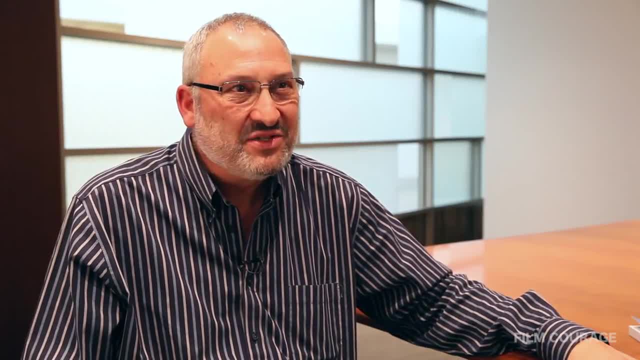 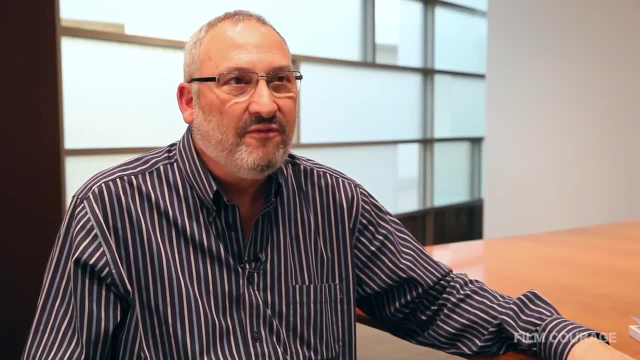 What if this happened? And that's a lot of where story ideas come from. That's a question I get. I thought: where do you get your ideas, Dr David Goldstein? Well, I have a lot of ideas from and I give an example of: I wrote family television shows. 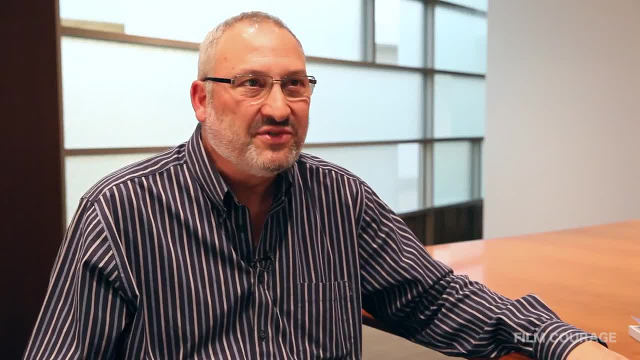 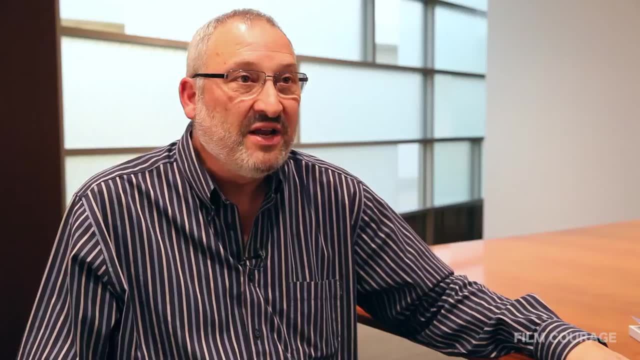 needed to write an adult spec script to show that I could write for adults. So I was going to write for Frasier Didn't have an idea yet, I was just living my life. My wife is a therapist And at that time she was a trainee. She had just gotten her graduate degree and was a trainee in an office. 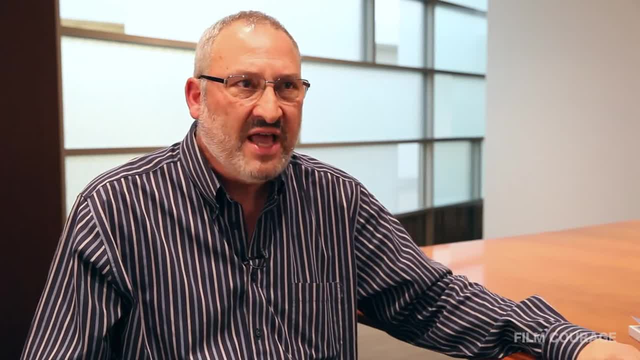 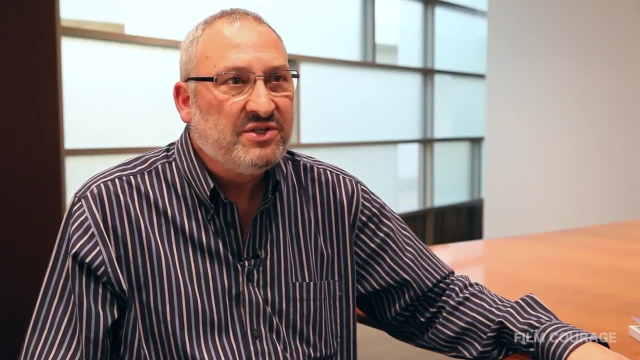 of therapists And the woman who ran the office- the head therapist there, had a Christmas party. So we went to the Christmas party And this at this woman's office. she had a Christmas party And this woman's area of specialization was she was a sex therapist, She was not a surrogate, She.